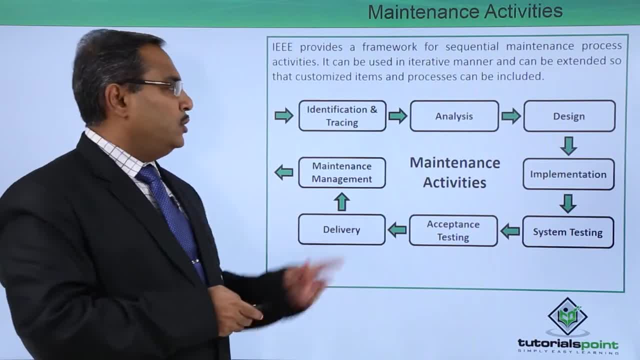 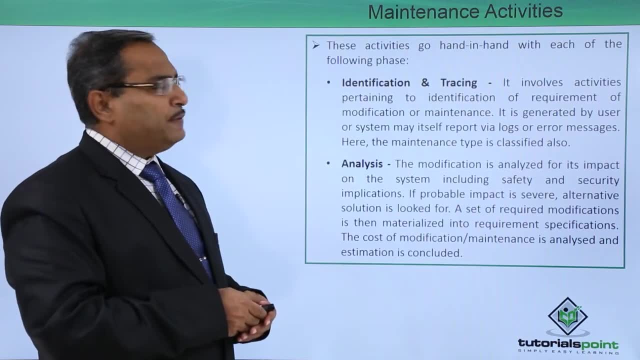 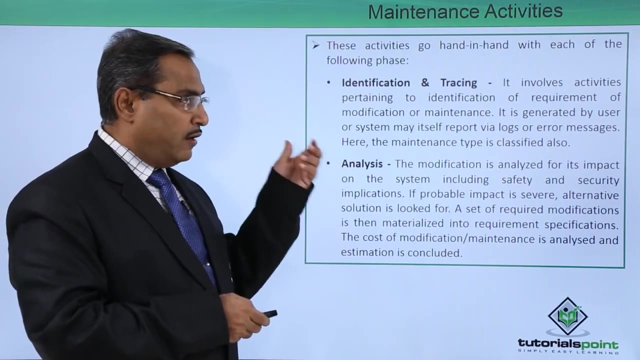 And we shall be having next maintenance management. So these are the different phases are there, So let us discuss one by one. So at first we are starting with this identification and tracing, So it involves activities pertaining to identification of the requirement of the 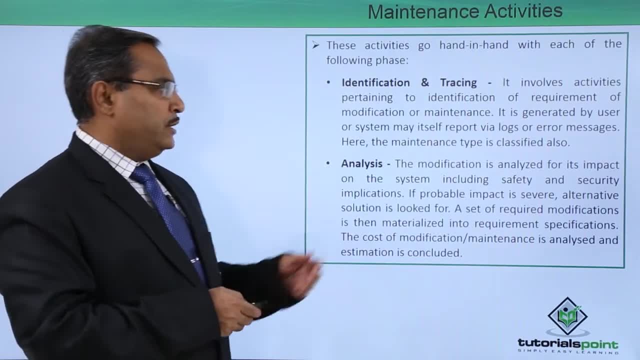 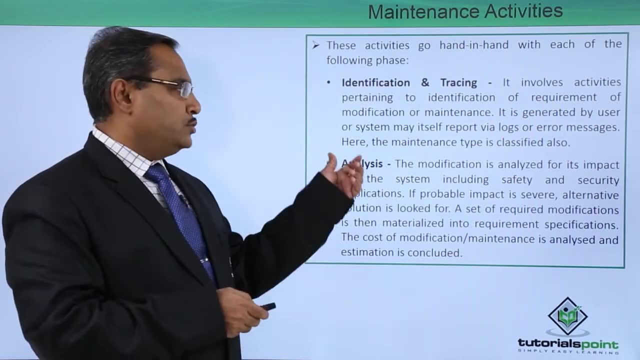 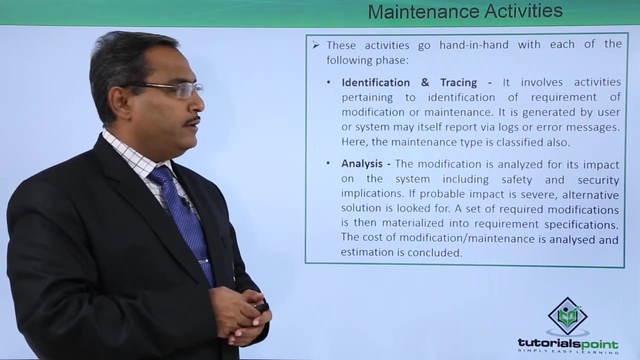 modification or maintenance, So it is generated by the user, or system may itself report via logs on error messages obtained. So here the maintenance type is classified also. So in this particular case, in case of identification and tracing, this particular request will be generated by the users and that will be. 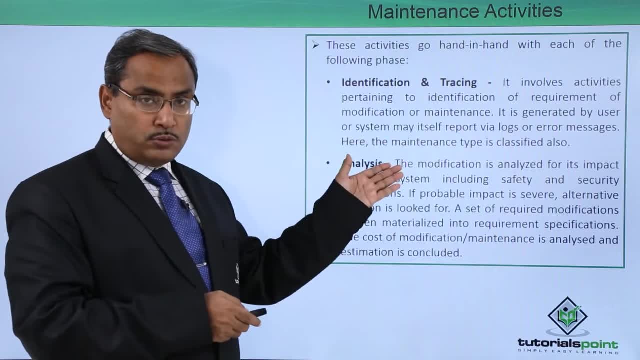 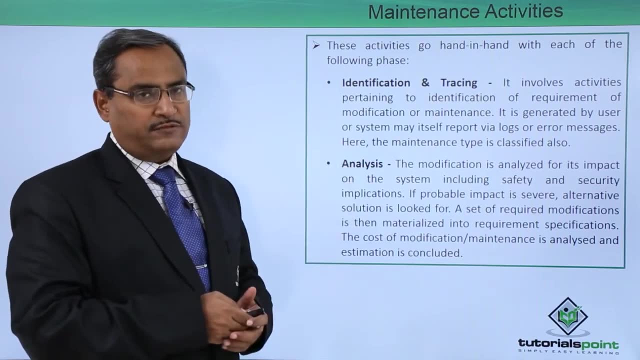 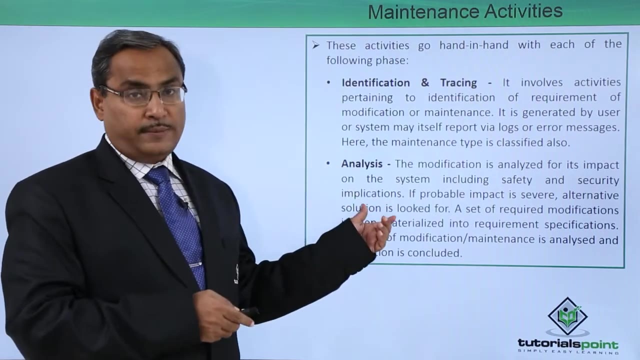 verified by the respective error logs and the error report And in this particular phase, this particular maintenance type will be also categorized or classified. Next one is our analysis. The modification is analyzed for its impact on the system. So if we carry out the respective maintenance required, then what will the impact on the 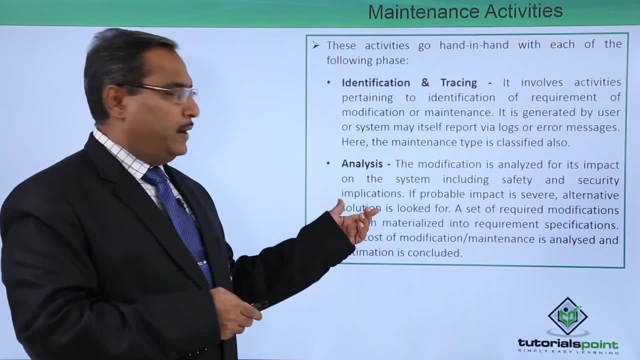 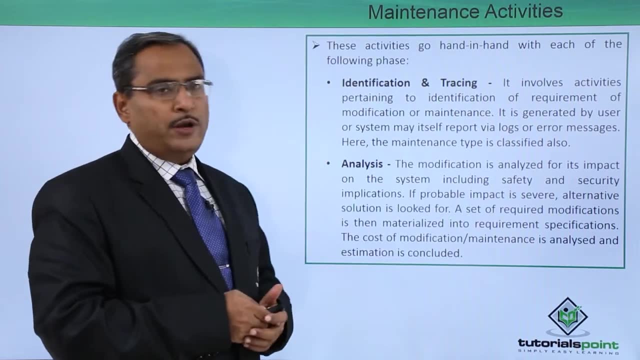 system, including safety and the security implications. So if portable impact is severe, and then in that case alternative solution will be looked for. And if we find that if we carry out the strict maintenance activity on this particular system, but the effect 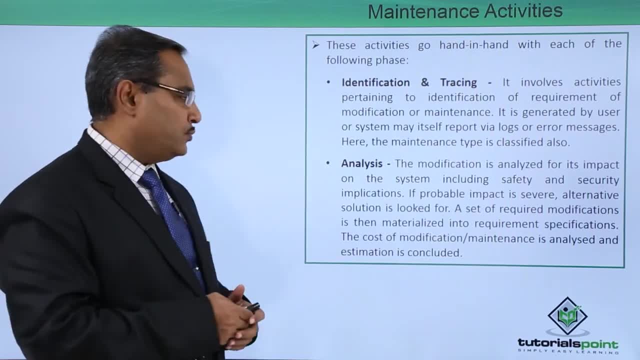 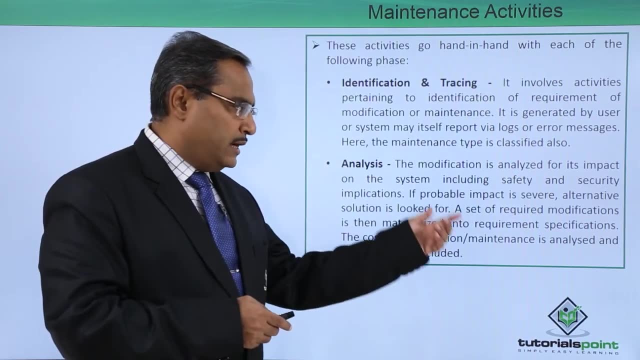 will be severe, then in that case we shall look for some alternative also. Then a set of required modifications is then attributed to the respective solutions. that is required. incidents related to the maintenance or BIB server cleanly put the maintenance activity materialized into requirement specifications. Now you see this particular maintenance requirement. 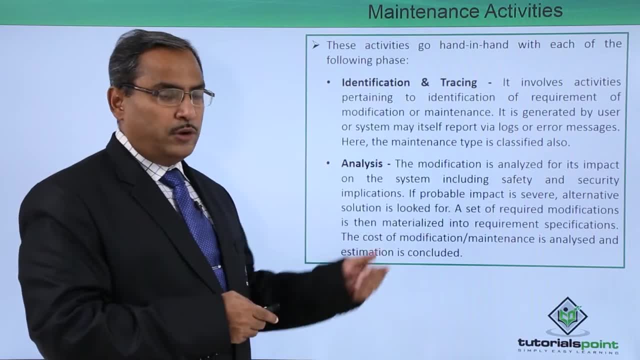 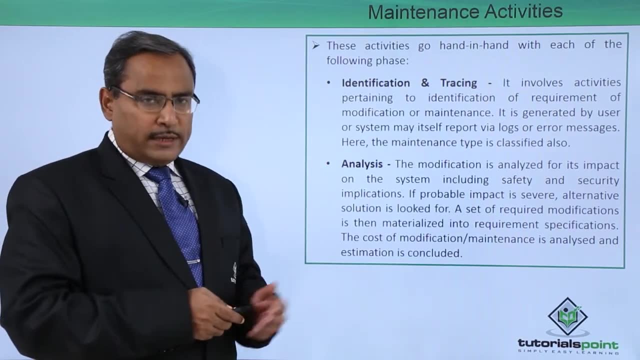 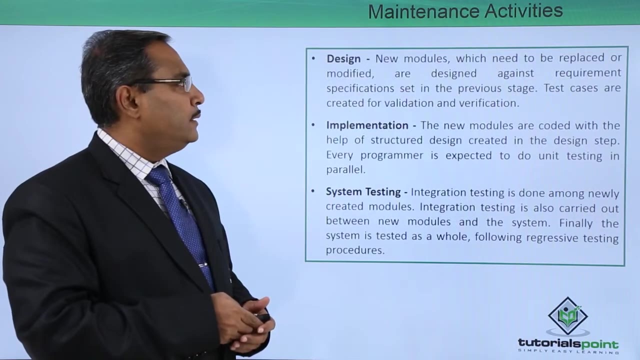 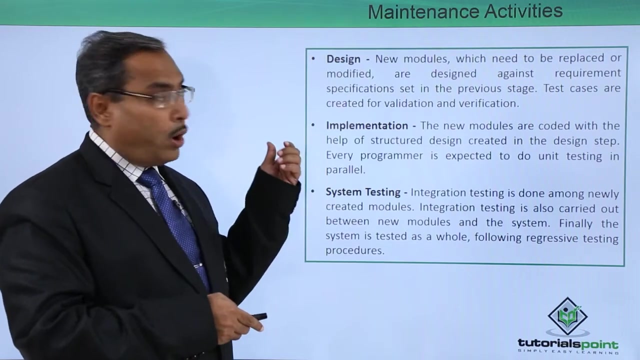 will be generated and requirement specifications will be also mentioned. The cost of modification, maintenance is analyzed and estimation is concluded. Estimation means the cost estimation will be concluded, So that will be done in the analysis phase. So next one is our design phase. So new modules which need to be replaced or modified. 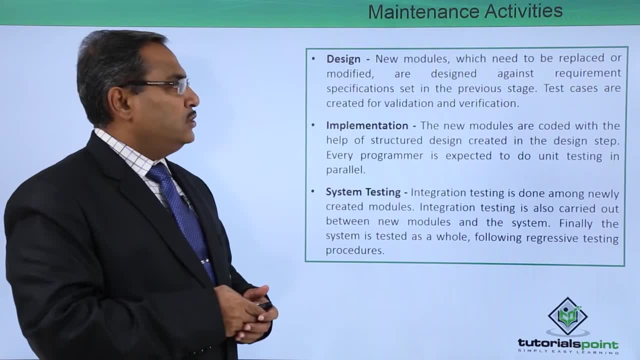 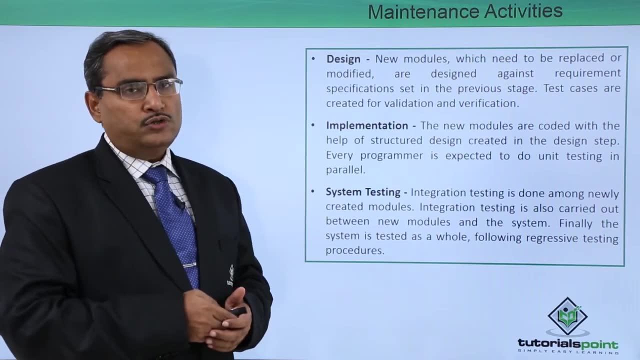 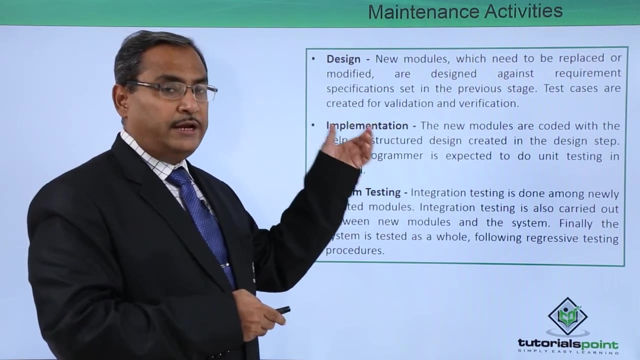 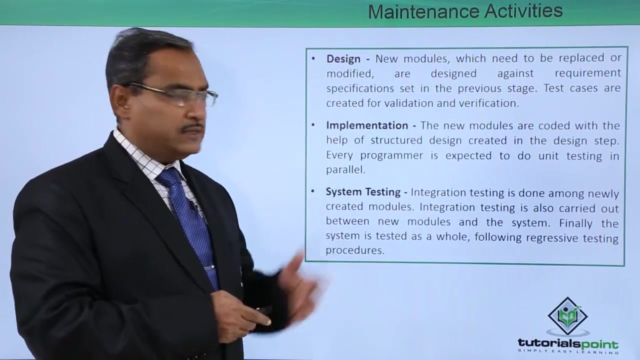 are designed against requirement specifications So set in the previous stage and test cases are created for validation and also for verification. So here in this case, in this particular design phase, the verification and also the validation will be done against the requirement specification set which we got in the previous stage. 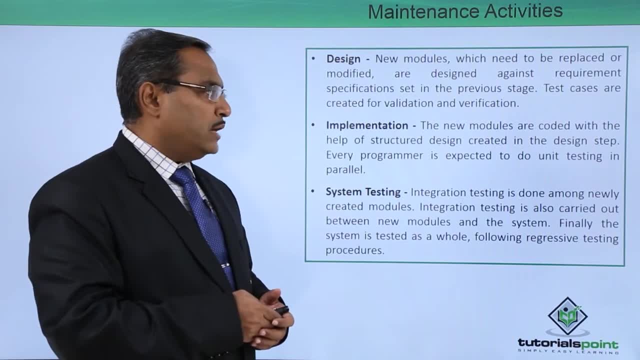 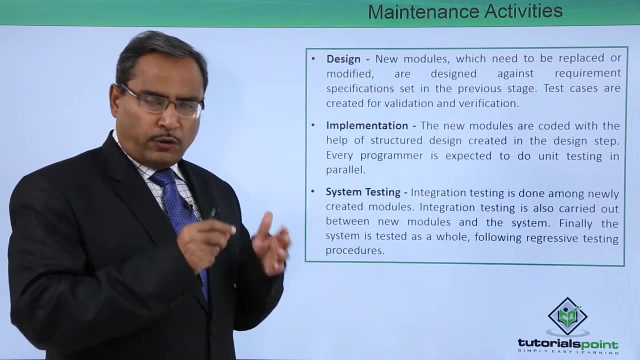 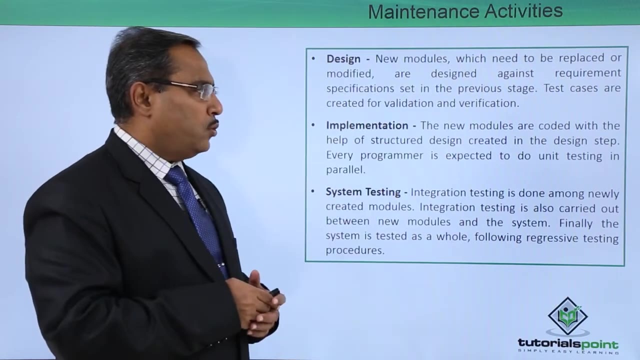 Next one: we are going for the implementation, So the new modules are coded with the help of structured design and created in that design step. So now we are going for the coding for the actual implementation of the maintenance process, So the new modules are coded with. 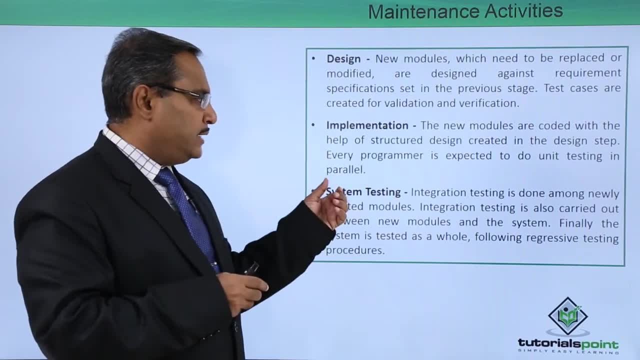 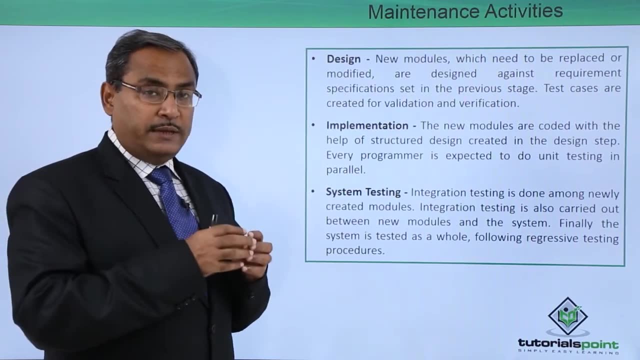 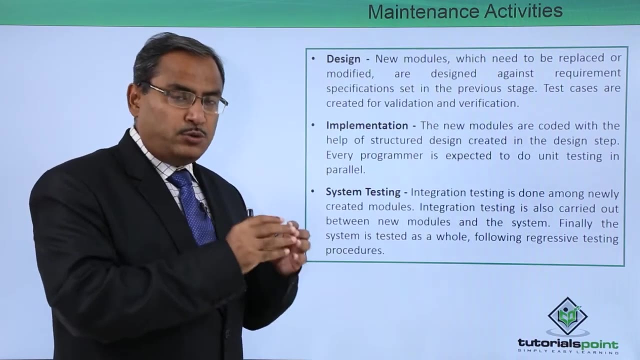 help of the structured design created in the design step and every programmer is expected to do unit testing. Subtitles by the Amaraorg community: testing in parallel. So unit testing means that very module which will be generated or the set of modules which are going to be generated, Each and every module, each and every unit. 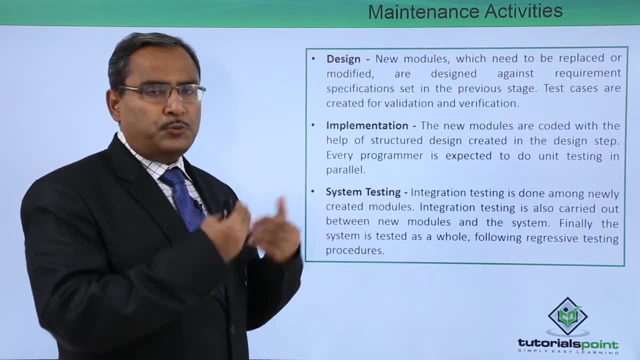 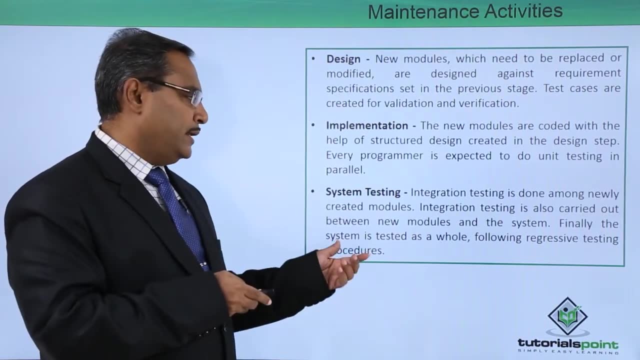 will be tested individually. giving certain set of inputs, outputs will be obtained and that will be matched with the expected output. So in this way the unit testing will be conducted. Next we are going for the system testing, So integration testing is done. among newly: 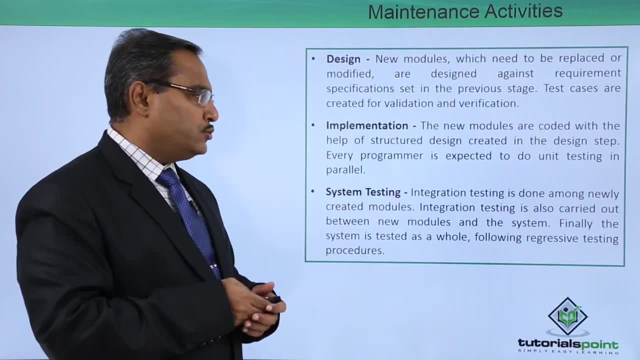 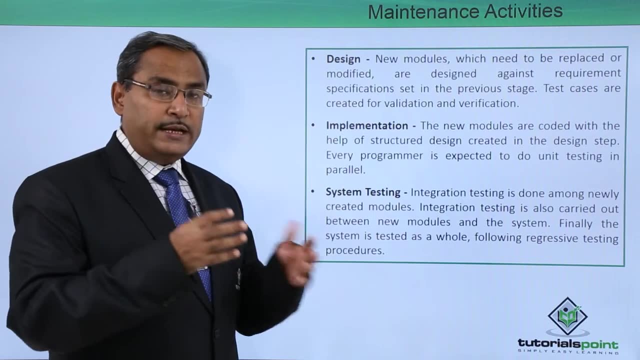 created modules. So now integration testing is also carried out between new modules and the system. So this new modules will get integrated with the system. So whether this integration is working fine or not, whether this pre-existing modules and this new module, 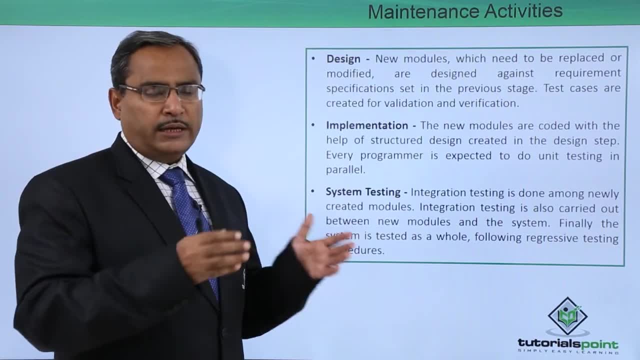 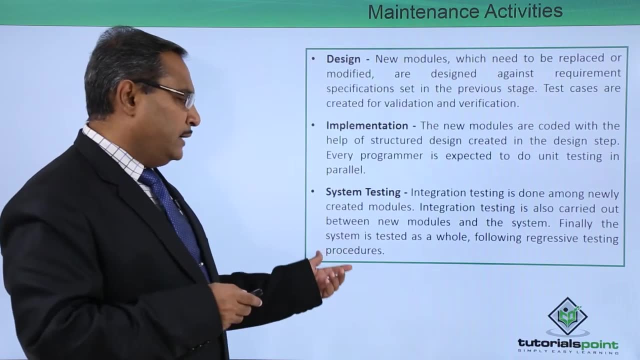 which has been developed for this maintenance purpose. whether the communications are done properly, whether they are getting integration integrated properly or not. that will be tested here. So, finally, the system is tested as a whole following the regression. So regression testing procedures. So you know that in case of regression testing, but 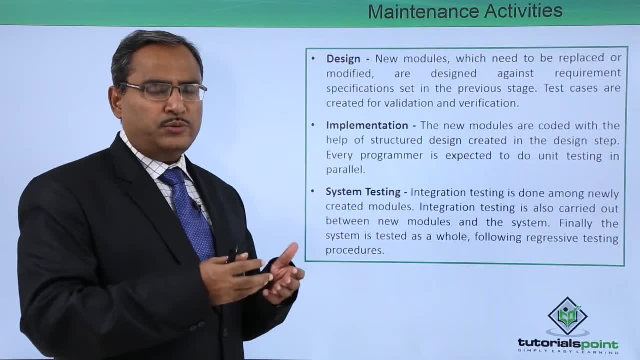 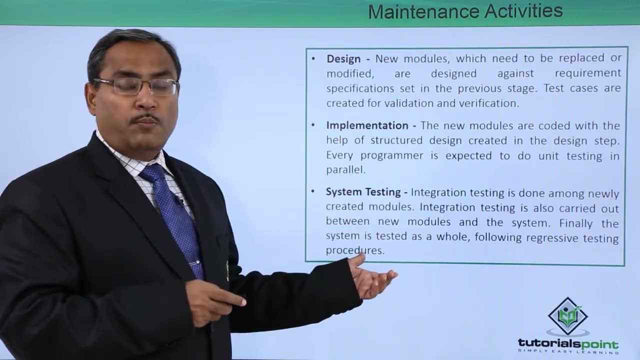 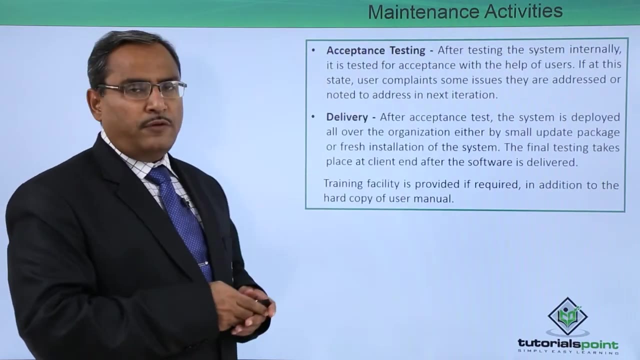 having some existing system and we have. for the maintenance process we used to include some new code, new module there and the regression testing will be checking whether this new module introduction is leaving some bad effect on the system or not. Next one: we are going for the acceptance testing. So after testing the system internally, it 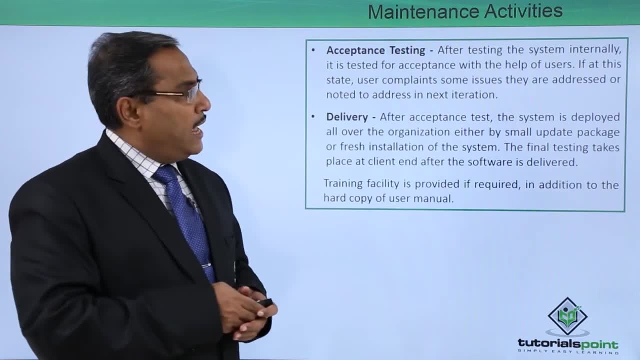 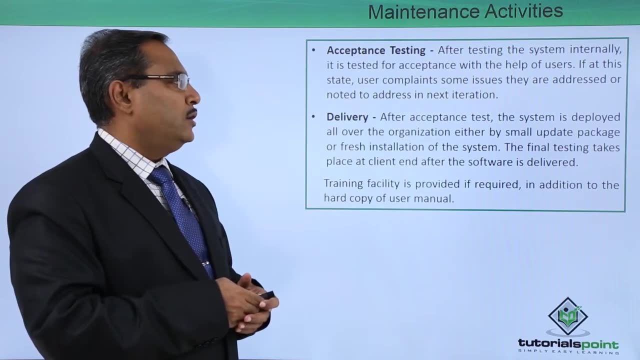 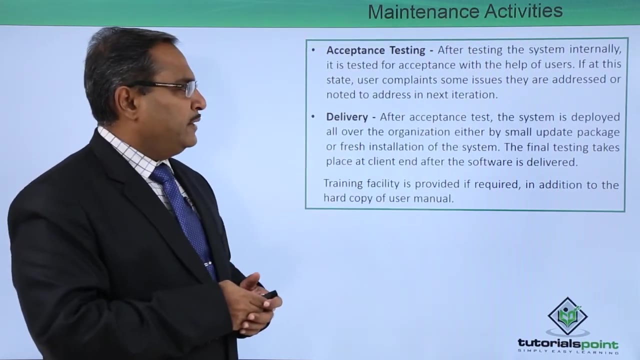 is tested for acceptance with the help of the users And if, at this particular state, the user complaints some issues, they are addressed or noted to address in the next iteration of the framework. Next one is the delivery After acceptance test. the system is deployed all over the